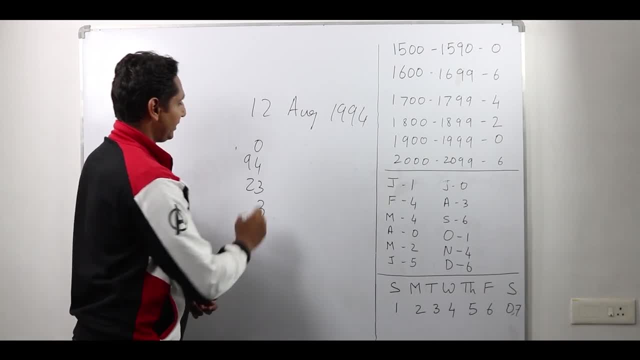 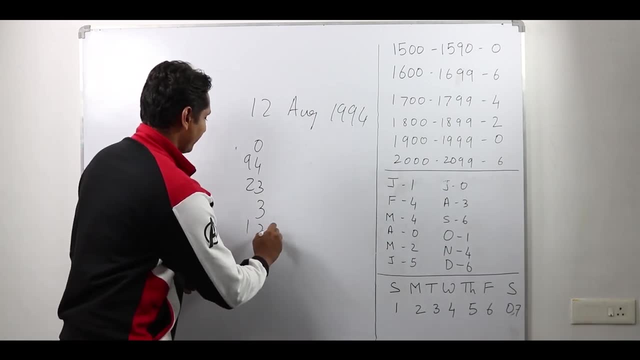 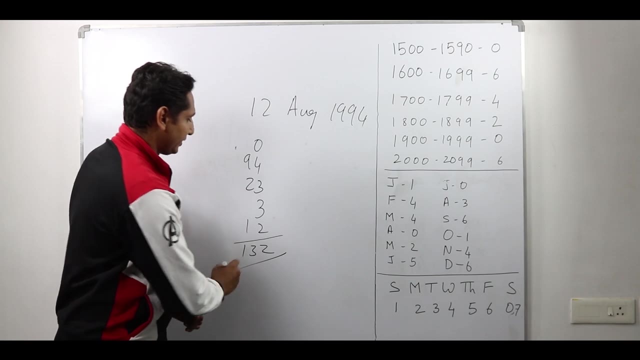 Code for August is 3.. I write 3 here. Okay. finally, it is the day which is 12.. I write that. Okay. now I have to sum all this, which comes to 132.. And this has to be divided by 7.. 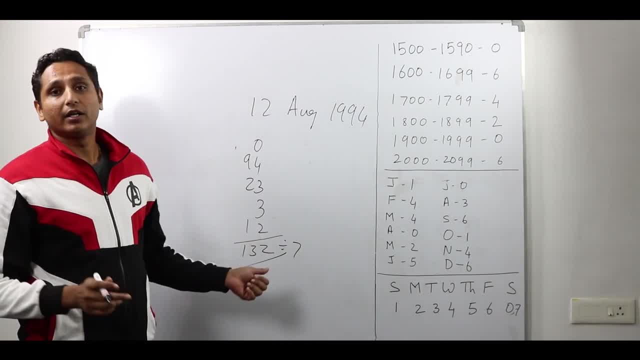 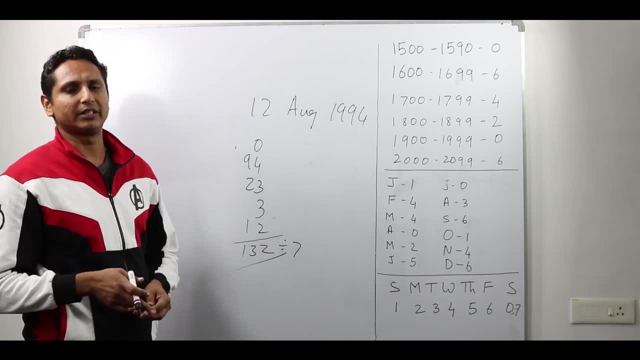 Okay And check what the remainder is. Okay. so in this 132, I remove 70,, 62 remains, which is one short of 63. So the remainder here is 6.. Now, what is the code? What is the day for 6?? 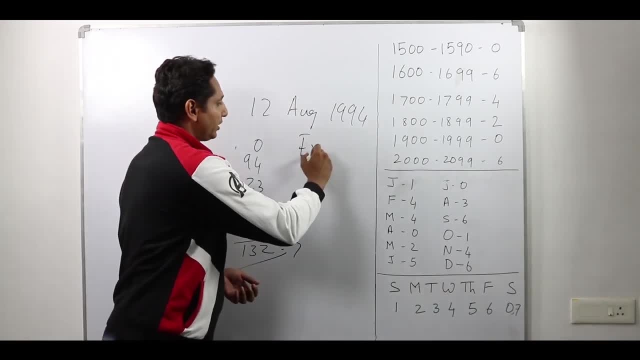 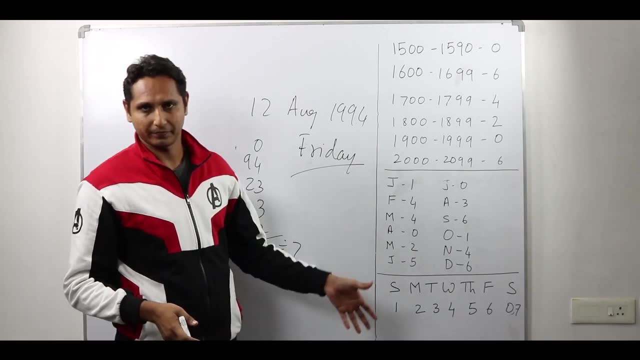 It is Friday. So 12th August 1994 was a Friday. Now I will quickly explain how these codes work. Okay, and how do you remember? Okay, now look at the years part. Okay, there is a pattern here. 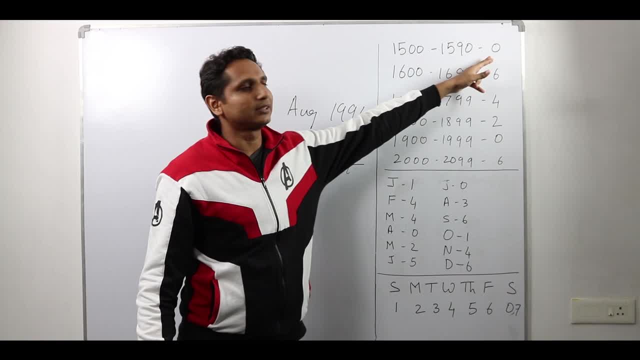 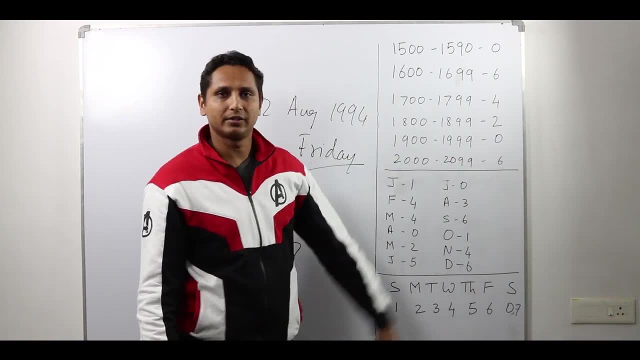 Okay, starting from 1500 to 1590.. Okay, it starts with 0.. After which it is 6,, 4,, 2, and then it repeats: It is 0, again, 6.. Okay, so this way you can remember the code for the centuries. 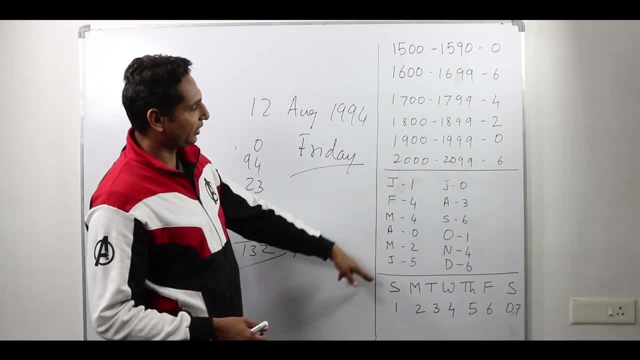 Alright, next is the months. So January, February, March, April, May, June, July, August, September, October, November, December- How do I remember this? So 144.. So 4 is 12th square. 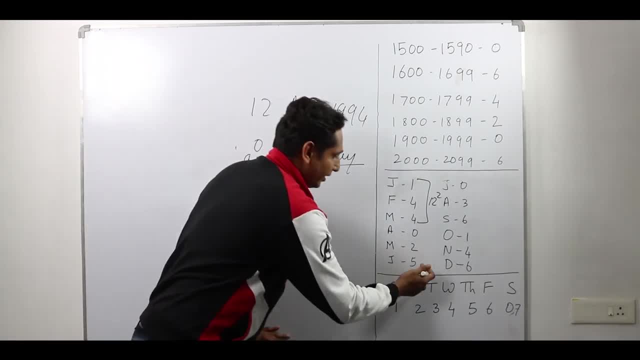 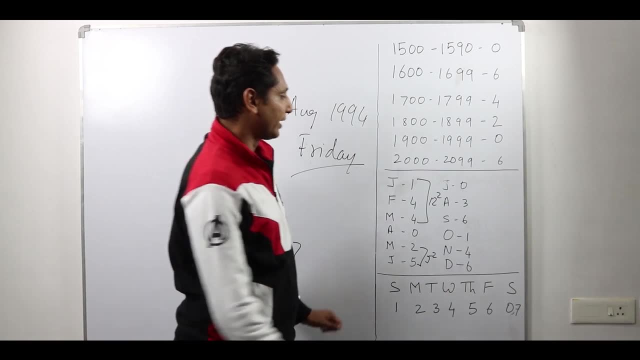 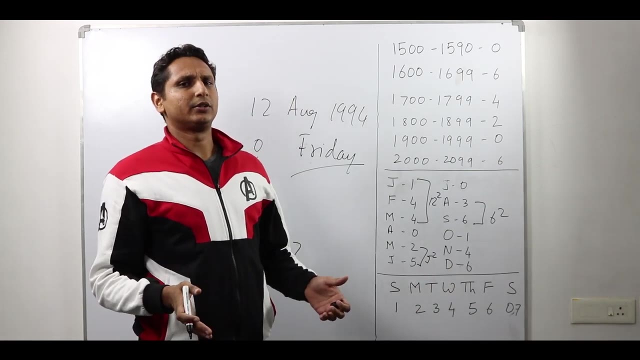 Yes, April is 0.. 25 is 5 square, Okay. then it is 0 again. 36 is 6 square, Okay, 146, I can write it as 12th square plus 2.. Right, So this is 12th square plus 2.. 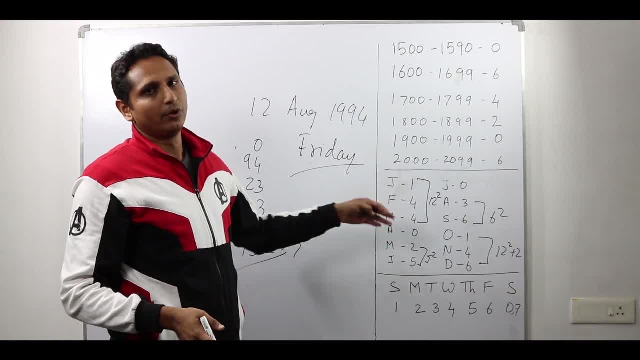 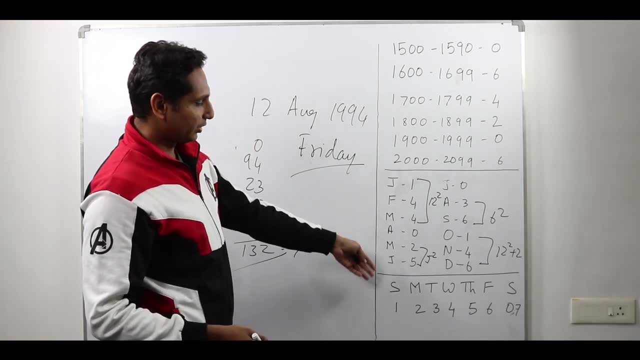 So this is how I remember. I remember 12th: 12th square, 0, 5 square, 0, 6 square, and then 12th square plus 2.. Okay, and about the days start with Sunday. 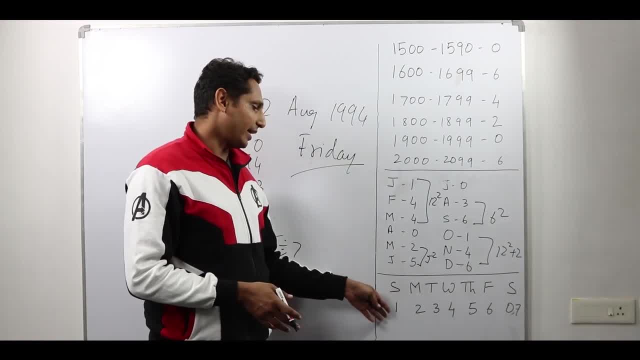 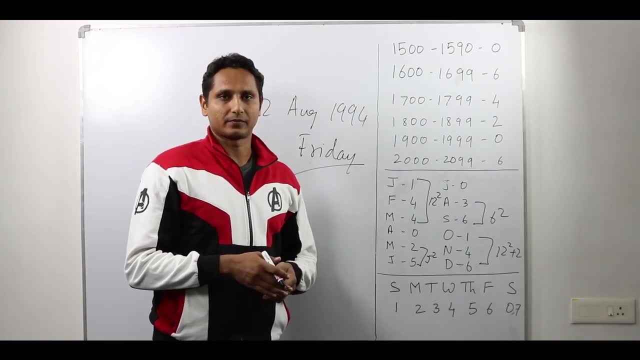 This is Sunday, by the way. Okay, so have Sunday as 1.. Okay so, and then move further Whenever you do not get a remainder, whenever the remainder is 0 or 7, which means 0.. Okay, the day will be Saturday.